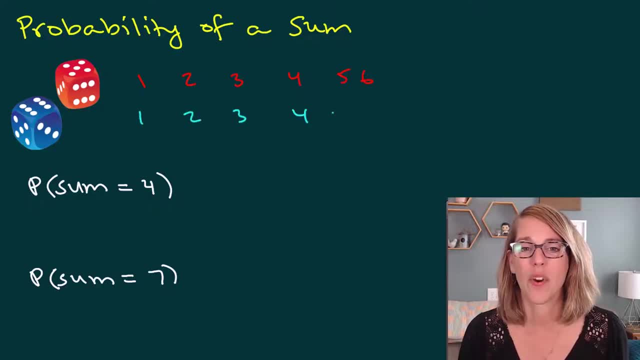 for that blue dice One, two, three, four, five or six. I also need the number in my sample space. This is the total possible outcomes. So the number in my sample space I've got six for the first dice, six possibilities for the second dice. Six times six is 36.. Now let's get into our sums. 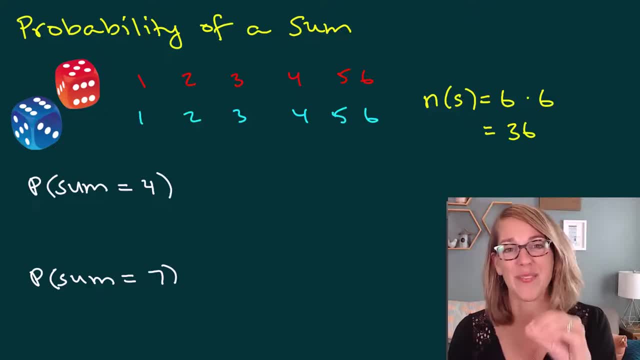 To come up with our sums. I want to put a number on the red dice together with a number on the blue dice to come up with some pairs. So if I want to add to four, I'm going to pair a one with a three. 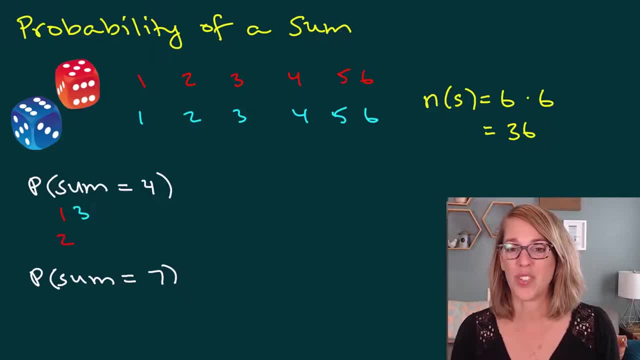 I could also pair a two with a two, So a two with a two, And then that one and three can also be swapped, and a three and a one, So I can also do a three and a one. So that leaves me with one, two, three. 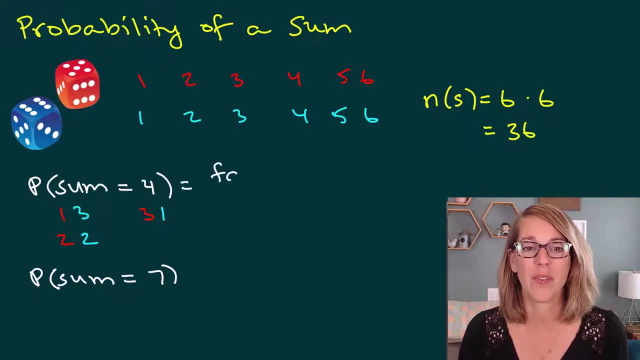 different possibilities. I'm going to put this together with my favorable outcomes. I'm just going to abbreviate favorable over total. I've got one, two, three favorable outcomes, So that's going to be three and a one. So that's going to be three and a one. So that's going to be three. 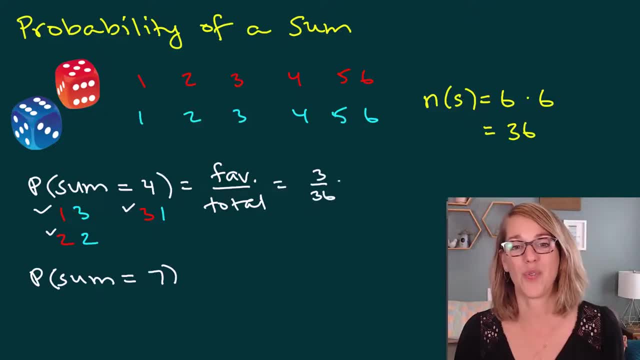 out of my 36, which I can reduce to one twelfth. Now let's go ahead and do the same thing with a sum of seven. I want to very systematically go through each of the numbers that I've got for my red dice and figure out how I can put them together with a blue dice to add up to seven. 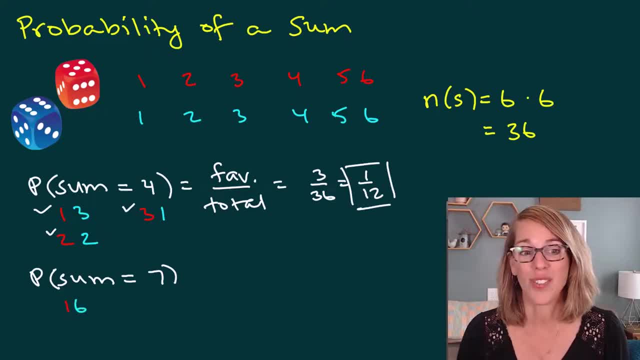 So that would be a one and a six. I could also do just going through the numbers here. a two would be matched with a five, A three would be matched with a four. I can do a four on the red dice and that would be matched with a three on the blue dice. Continuing. 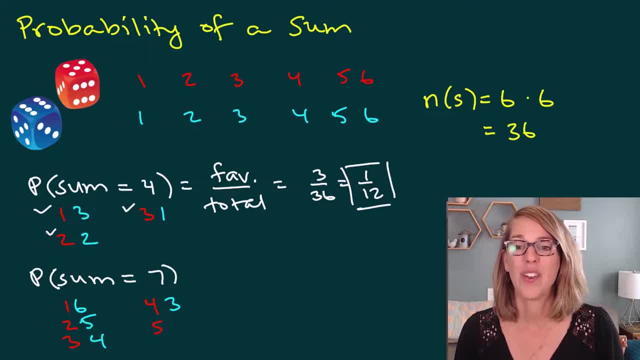 to count up here: on the red dice, a five would be matched with a two on the blue dice. And then, finally, I've got just one more way to do this, and that would be a six on the red dice with a one on the blue dice. Now I can make sure that I've got everything paired correctly by making sure. 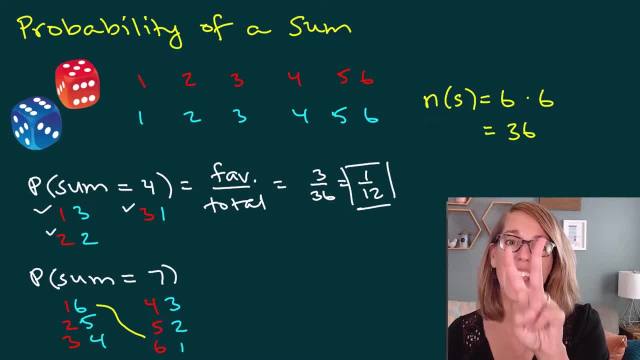 I've got those opposites right. A one and a six can also be paired with the opposite dice as a six and a one. They're all there. So that leaves me with one, two, three, four, five, six possible outcomes. So that would.